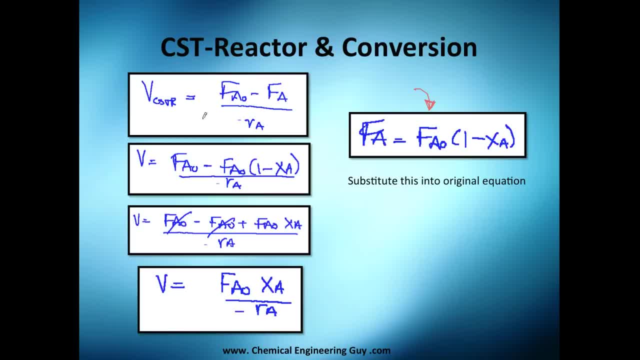 difference in conversion. So you know hopefully, by definition, this volume of the continuous-tiered tank is equals to F minus F divided by the rate of reaction. Now what will happen if we just literally plug this equation here? We will have F of A initial minus F of A initial. that 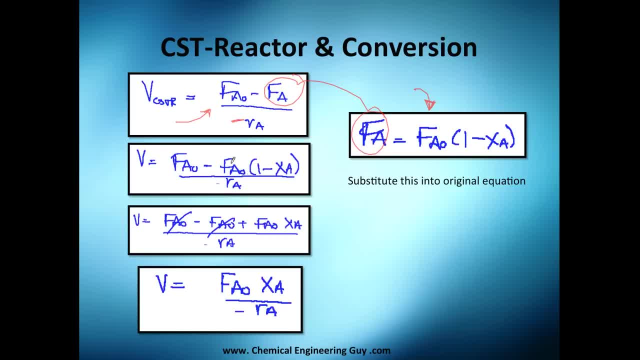 multiplies 1 minus X of A. Now let me develop that. You will have this times 1 and this times minus X of A. So I get rid of this, I get rid of this and I get this positive value here. And this be sure, don't forget this negative sign. and 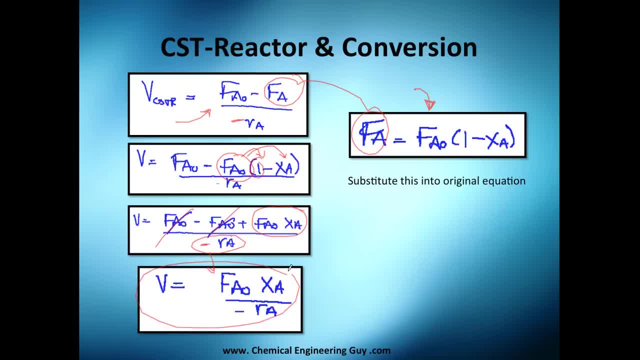 we drop it here And this is everything. guys, It's nothing that complex, You're done. You got a volume of CSTR or a continuous-tiered tank reactor, depending on the amount you are feeding or the flow times, the conversion you are achieving or you want to achieve, divided by the rate of 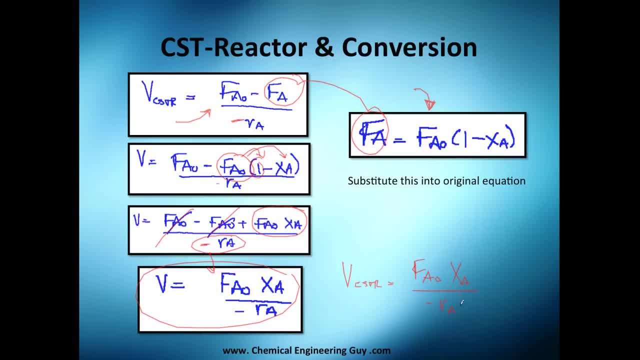 reaction and hear me very clearly at the outlets. So if you have a conversion of 80%, you need the rate of conversion at that 80%. So that's everything for the continuous tier tank reactor. we're going to see more examples later, so please don't be wondering: where are the examples? just wait a. 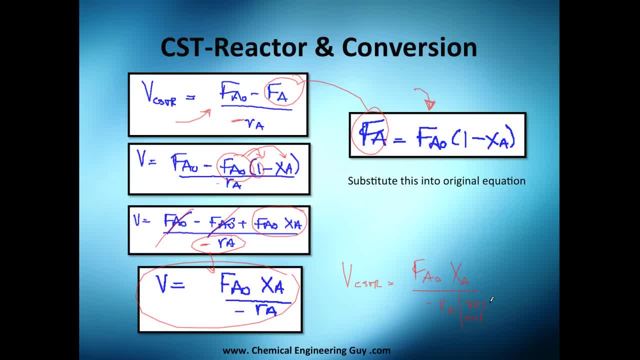 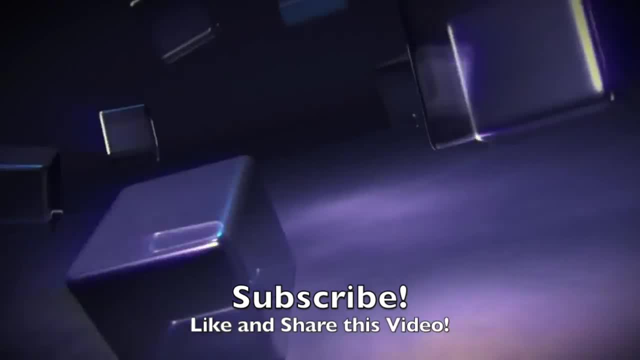 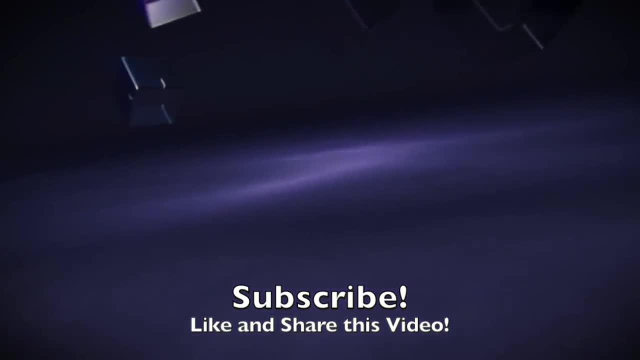 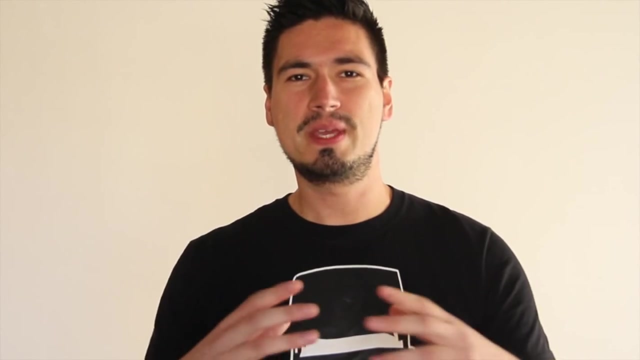 little bit. watch the other videos and we will be starting playing with these equations. What's up, guys? it's me chemical engineering guy. so if you like the video, why not push the like button? it really helps me to know if you're liking the videos or if i should be changing something. 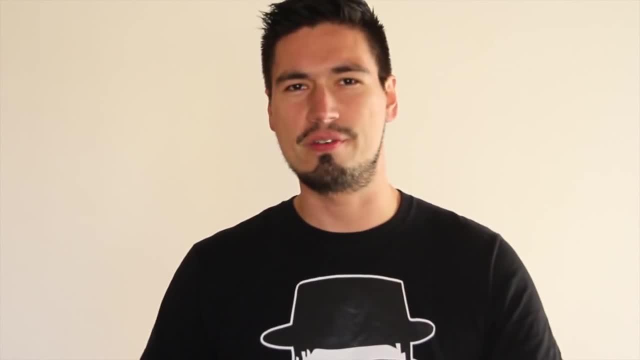 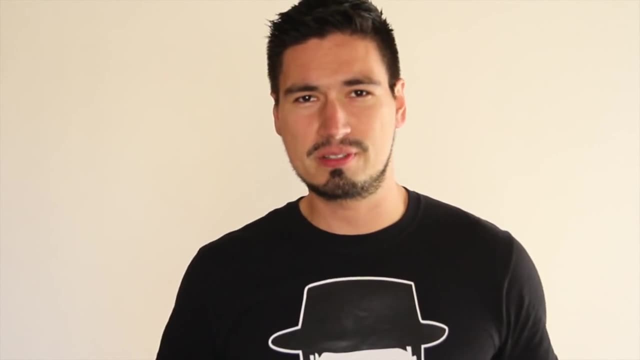 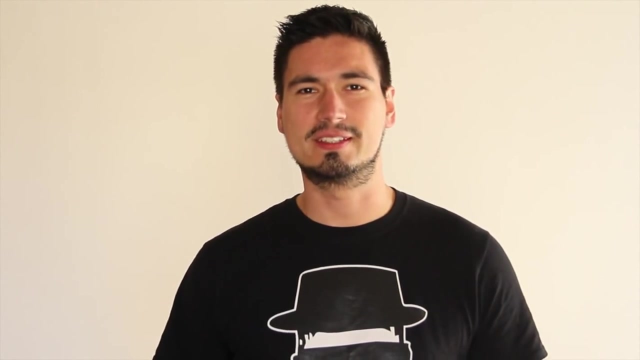 or i should be adding something, taking out content whatever. also, sharing is caring. so if you got any kind of friends, teachers, colleagues or whatever kind of person that might be interested in this type of content, why not share it? sharing helps our community to grow faster- in members and in content.